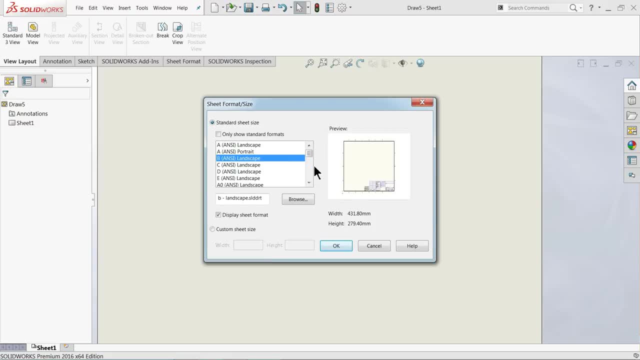 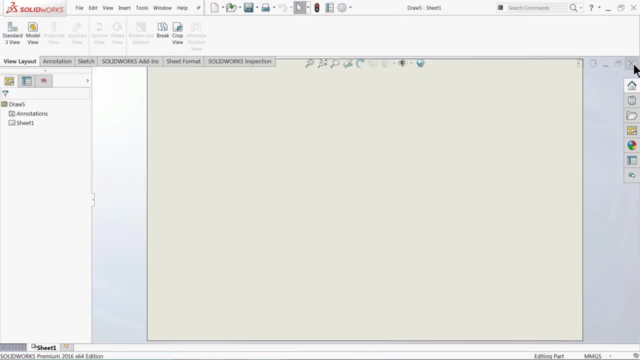 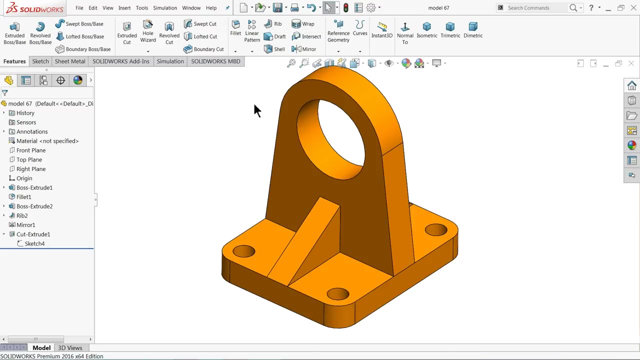 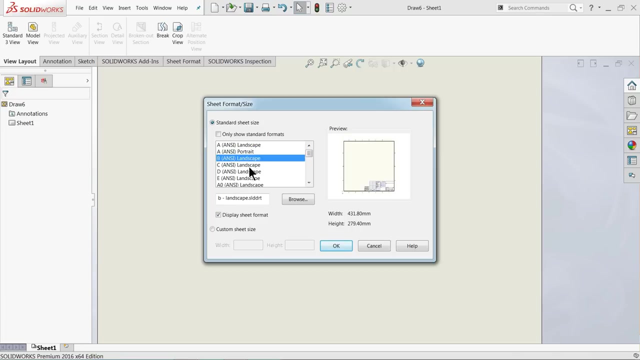 It will ask you your landscape, your size of sheet. So anything you can choose it. But this is the letter we will see. Cancel it. And the another way you can, directly entered from here: Make drawing from part assembly. Now see here: Any landscape size you have to choose. So I will choose here landscape B. 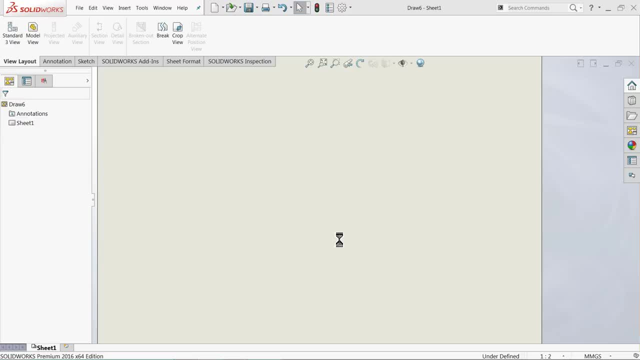 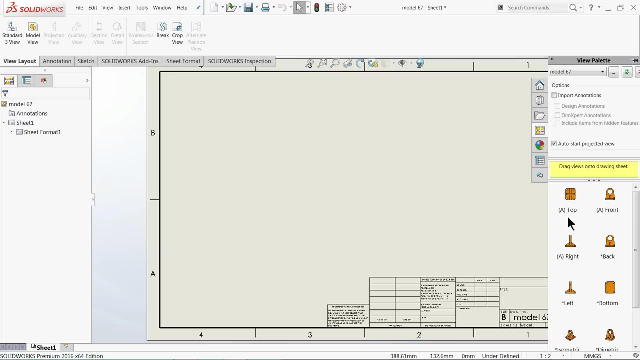 OK. Now, once you click OK, It will give you in your left hand side view palette. You will see there are multiple things, Multiple options. You have to choose any one and drag it. So I will start with front plane. I will start Drag it. 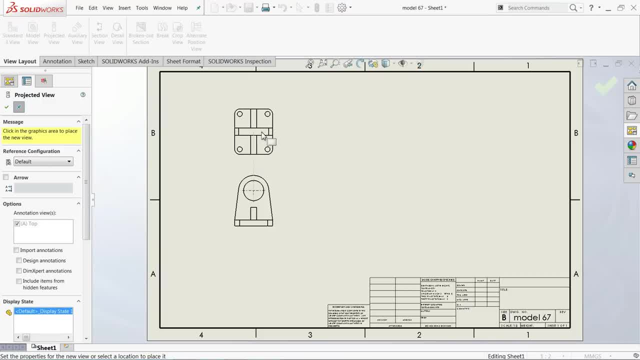 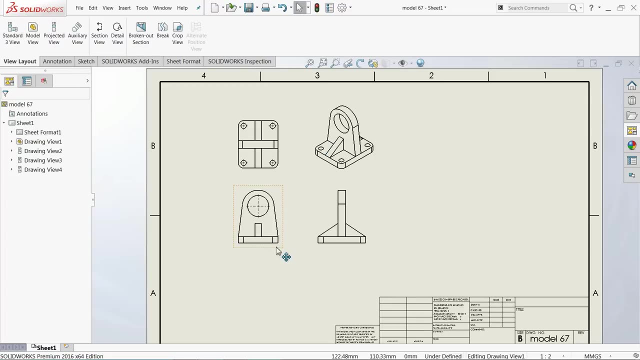 Then drag top side Top view And right hand side view, And if you want isometric view, you will see Here. click OK Now. even though if you like to increase your, This is your basic or first view Custom scale, Even though you can change the scale from here: See: 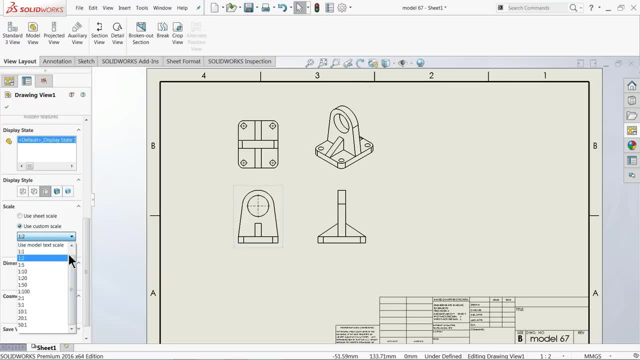 But that is OK, Even though you can choose from here: User defined 3.. It's going too small, So 1.5, that's fine, But 2, that's fine. OK Now, even though, if you like to change, Right click on sheet. 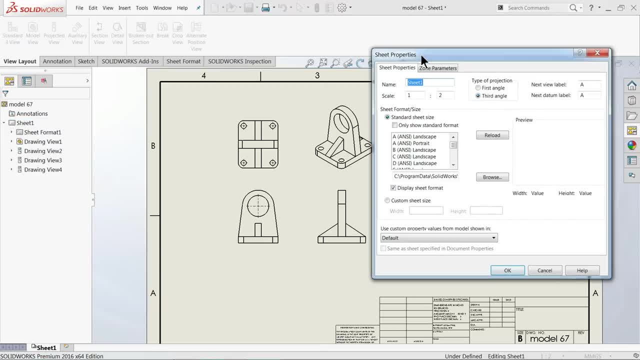 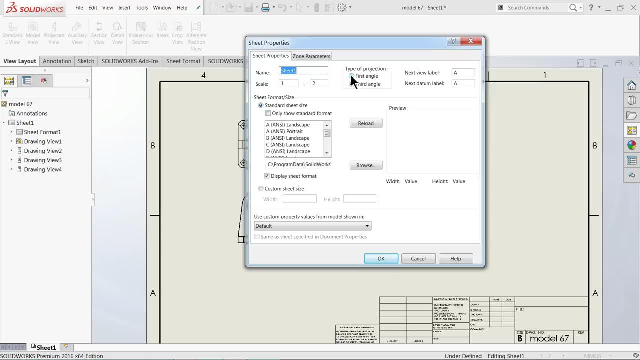 And here go to properties And from properties you can change the sheet name. Scale also you can change here 1 by 2.. And angle- Third angle- is the standard angle people going to choose. So I will keep third angle, Even if you can change. 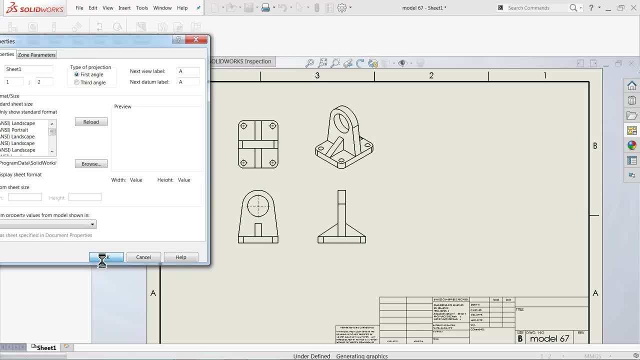 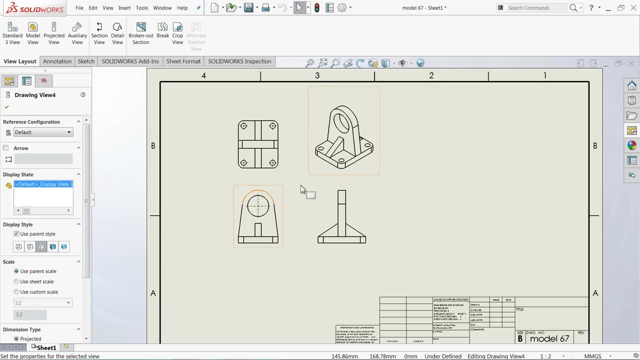 You will see first angle Now see It's changed, But we will keep third angle. This is the standard way. Now even You can choose individual color. So if We want to change this color Here, Uncheck, use parent, Because this is your parent. 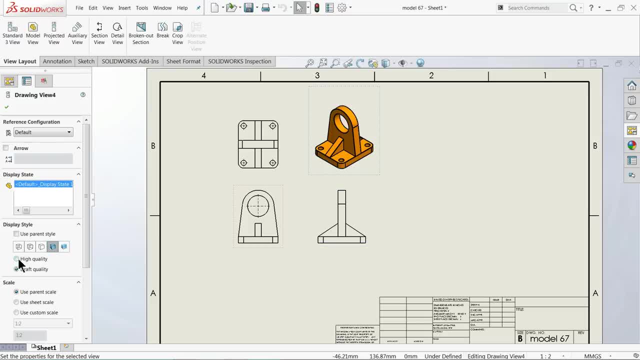 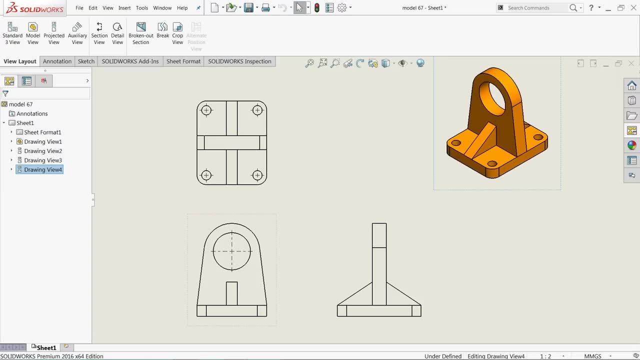 Styles: Now see individual. I can change. Keep high quality, That's it. You can drag it. Now this one Hidden line visible. Now you will see here, hidden lines are visible Even though we can define the Import annotations and dimensions from here also. 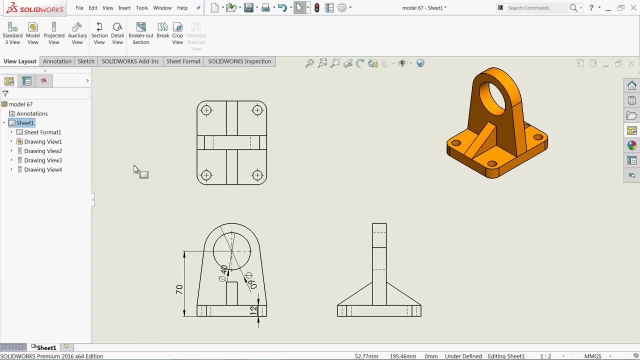 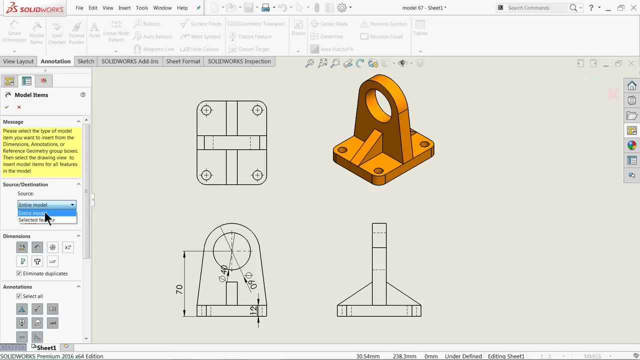 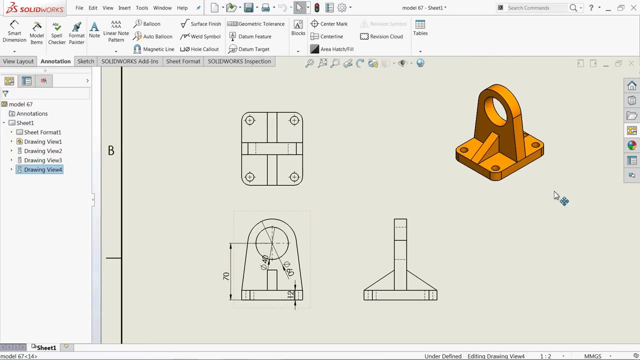 Or there are one more options, I will tell you. Or simply just Go to annotation model item And here choose entire model. But we will not do. We will do one more thing. Then we will apply Drawing in full view. First, we will see how to make. 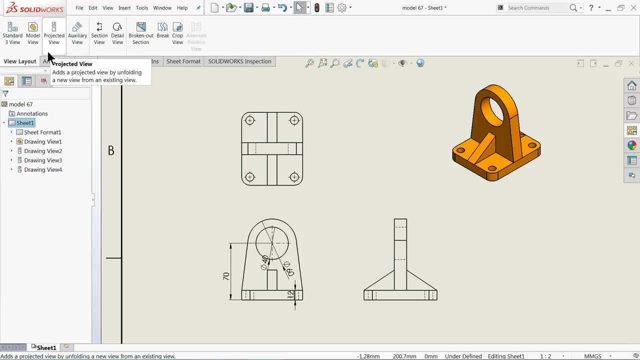 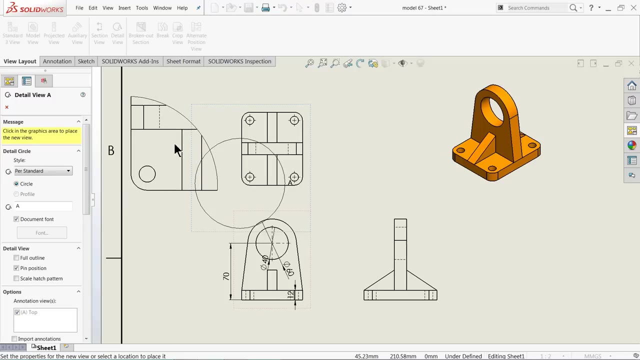 Now here one option: Detailed view Circle: Just drag Now see. Click Now. here you can define All the things. Even you can choose hatch Full outline, Even though you can choose Uncheck this parent and See. 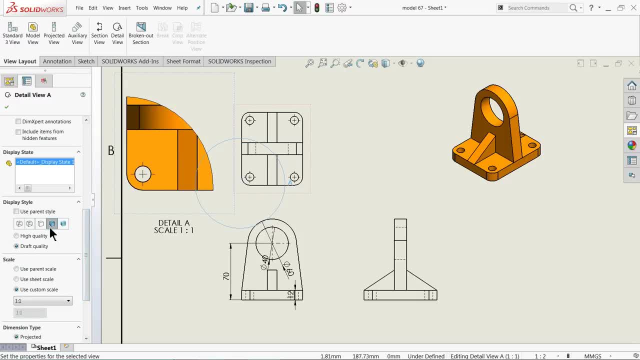 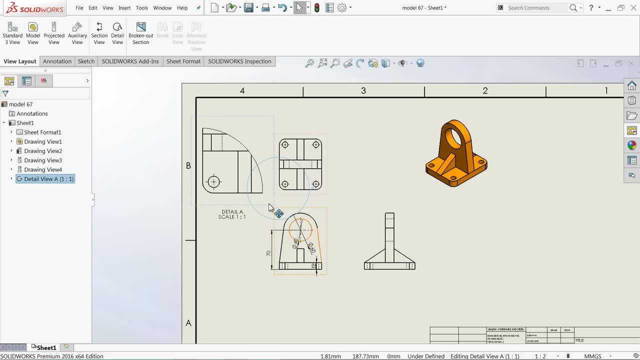 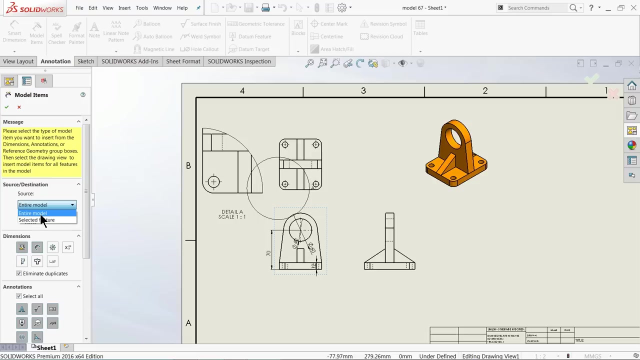 This color also, we can change, It's up to Us. Okay Now Model view Model item. Here you can choose entire Model And click all the things so that All the details will come here. Click okay Now see. 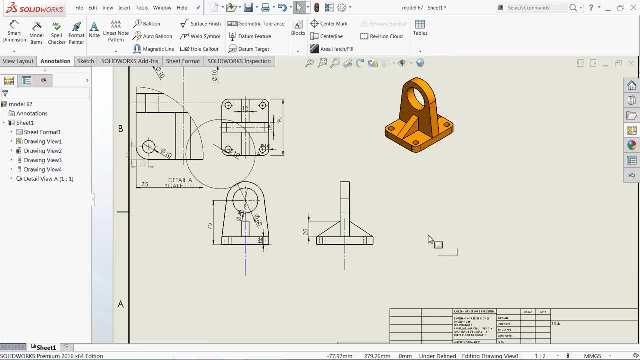 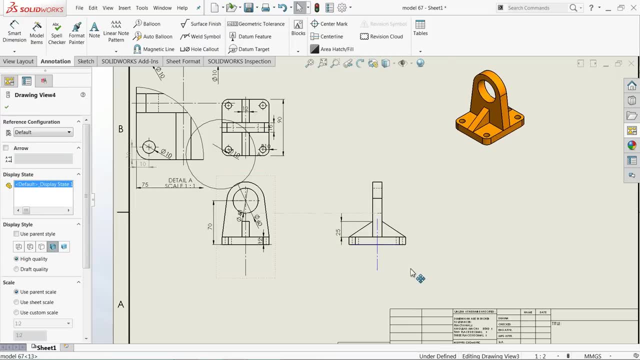 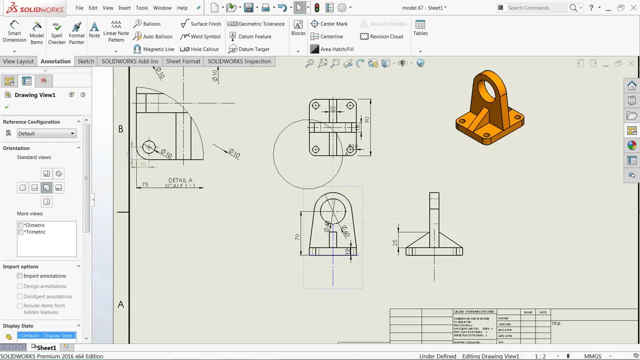 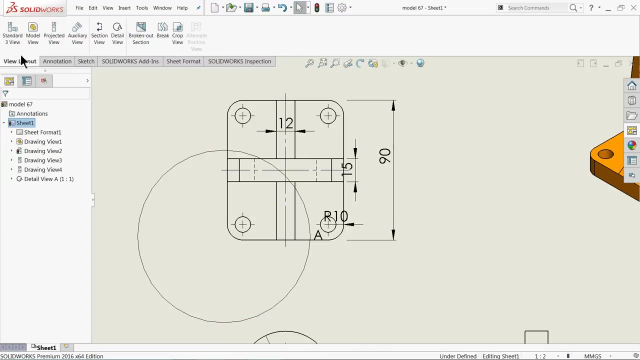 All the details comes here Now let me do one thing. Just arranged it Because it It seems To hustle and bustle. Now see, Even though you can apply, If you want to apply dimension Individually, We have option here in annotation. 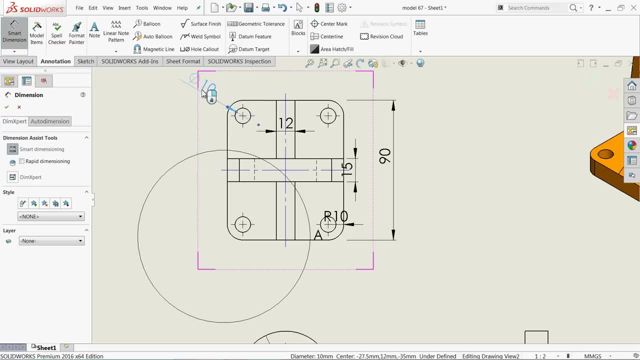 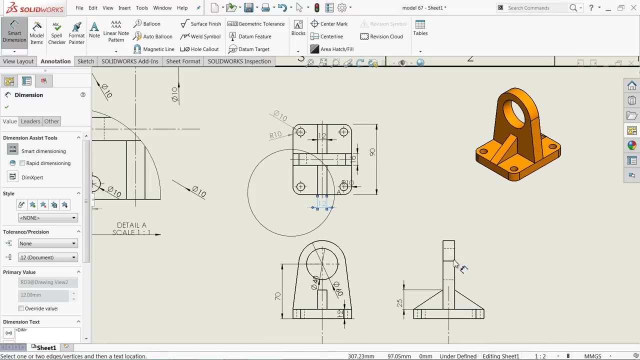 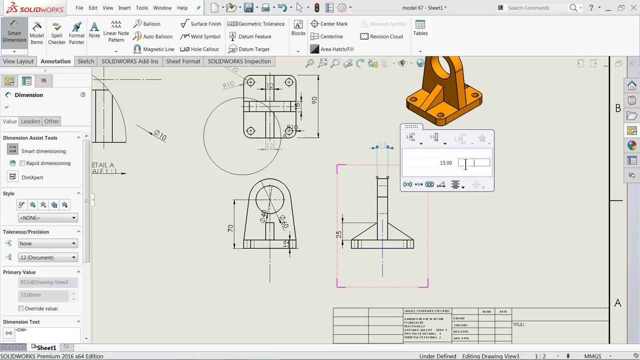 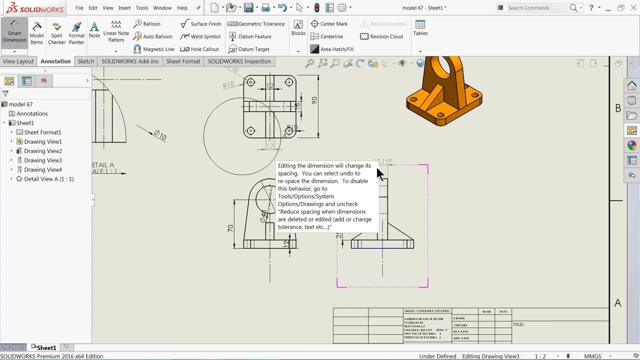 Smart dimension And you can assign A separate dimensions Or individual dimensions from here. See, If you click, You will see a small window. You can. You can Click here. Type A: typical dimensions. Now see Okay. 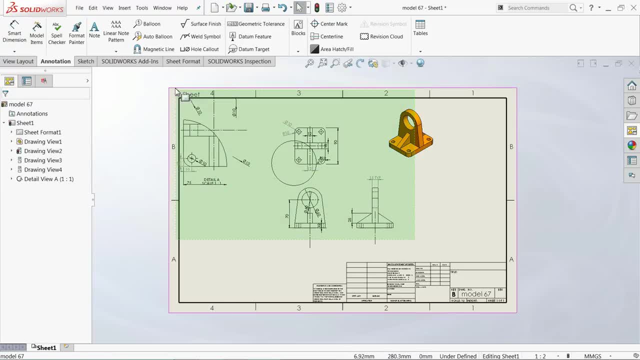 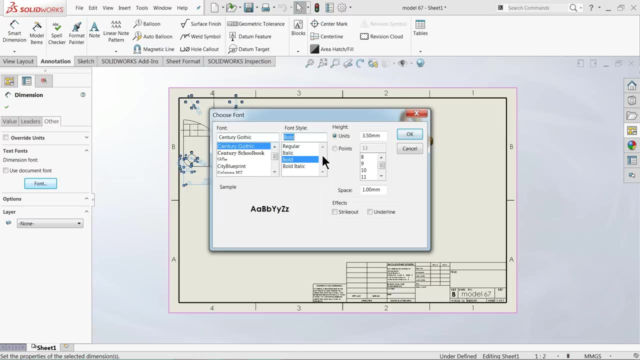 Even though if you Want to Make the dimensions Go to other, Use font, Uncheck font And from here We can change the size And Font Style, Everything from here. So I'll keep bold Size. 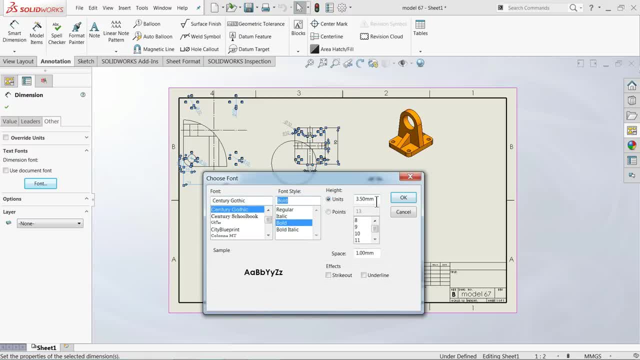 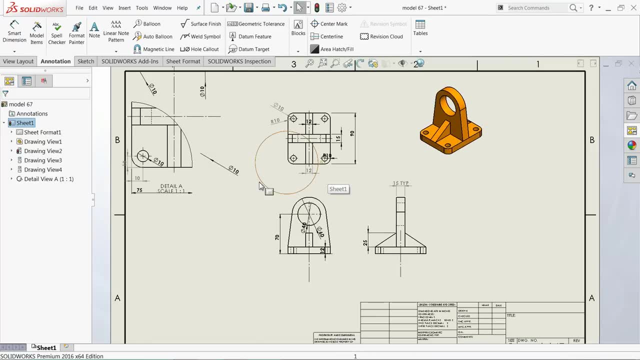 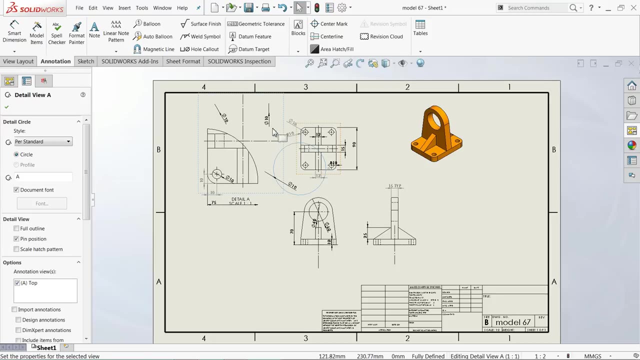 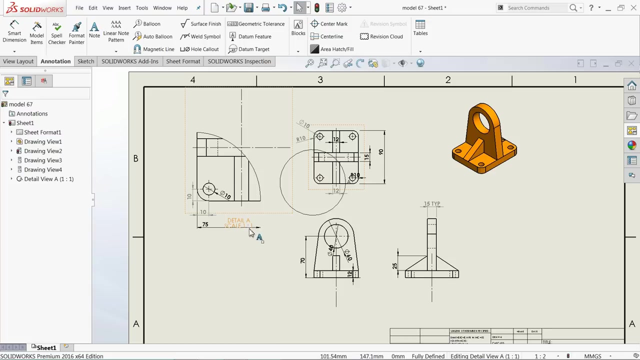 I feel that's Better. Or, if you like, You can make Formula, But bold is enough. Now look Now. this is the section view What we created, Those things you don't like, Just simply delete it. So this is the section one. 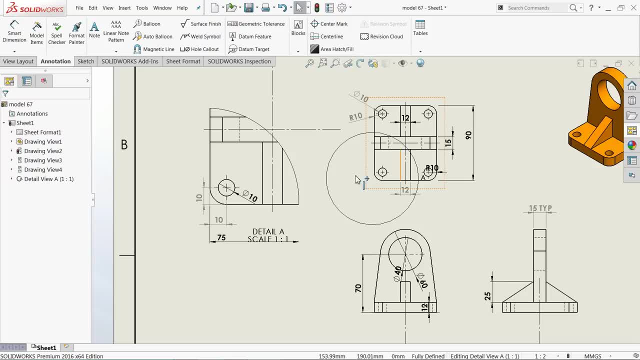 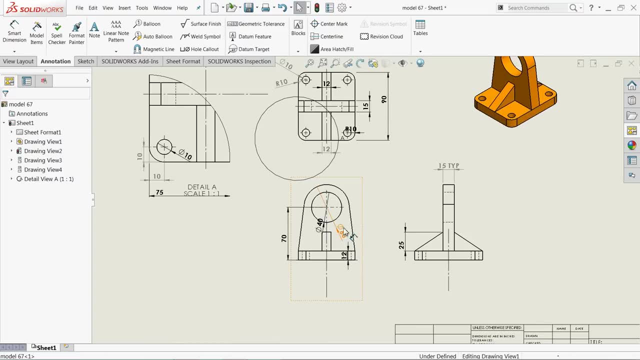 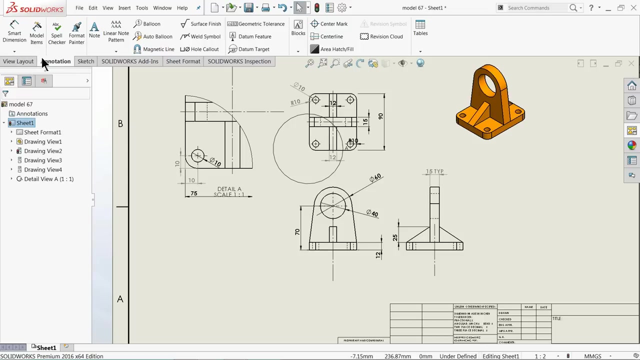 Here you will see A detailed view of this Circular part. I told you, even though You can change this one, Okay, This is your drawing. Even We have one more option here: Section view. If you go to section view. 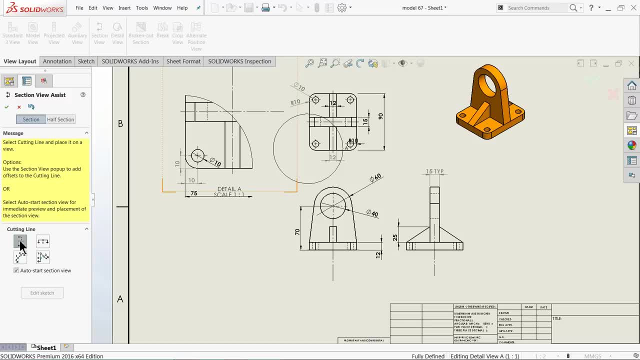 You will have multiple number of cutting. First We will see. If you drag, You will see. So you have to put your Cursor on the center And it will ask you Section view. Click Okay And you will see. 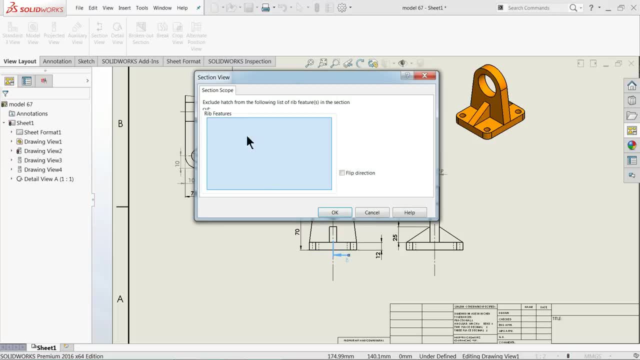 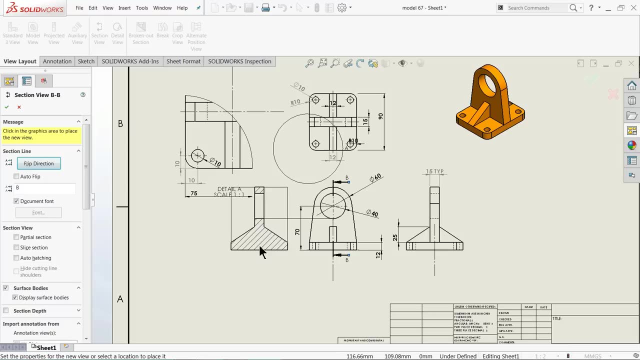 Drag in any side Wherever you like. So let me drag this side Now here You have Too many things- Documents For You You Want To Draw, So You Have This Documents. 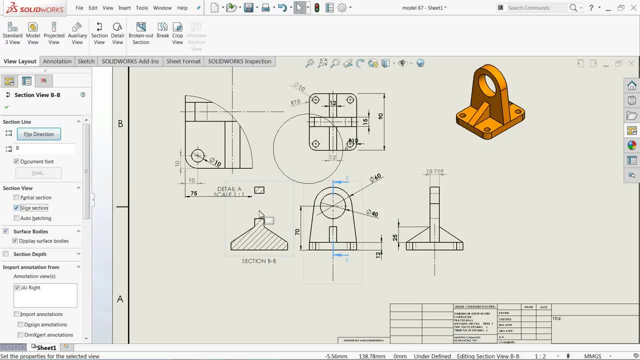 Font. That means The same font. We will keep Slice. See, If you Click Slice, Section The Only, It will Show You Shaded Portion. Okay, Now Even You.